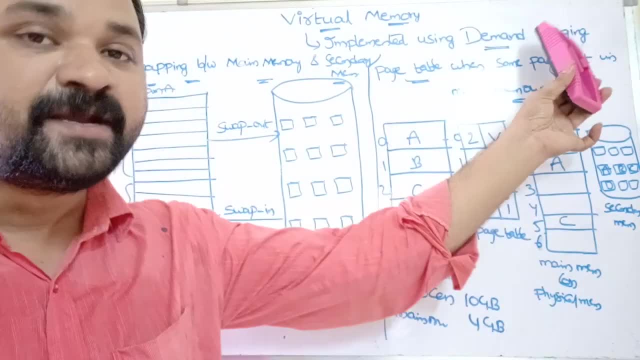 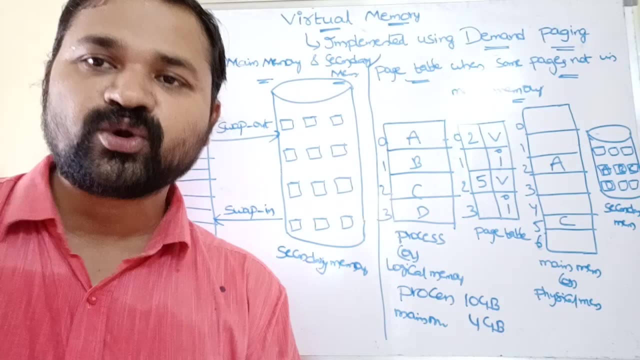 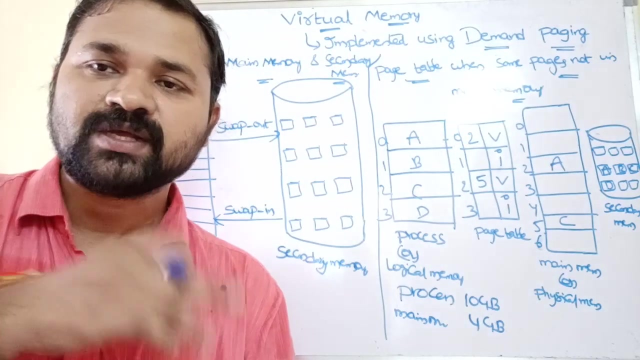 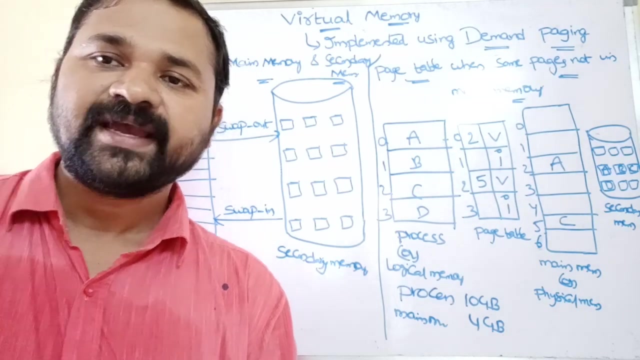 Virtual memory is implemented using demand paging. The name itself specifies the meaning. Demand paging is nothing but paging only. That means the given process or the logical address space of the process is divided into a number of equal size partitions called pages. Likewise, the main memory is also divided into a number of equal size partitions called frames. 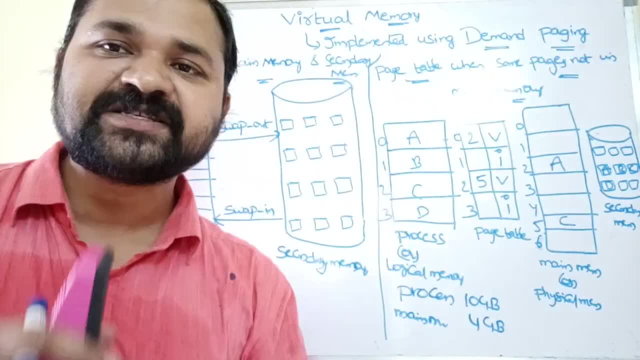 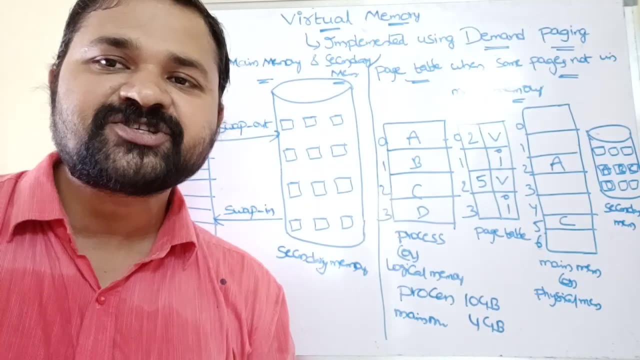 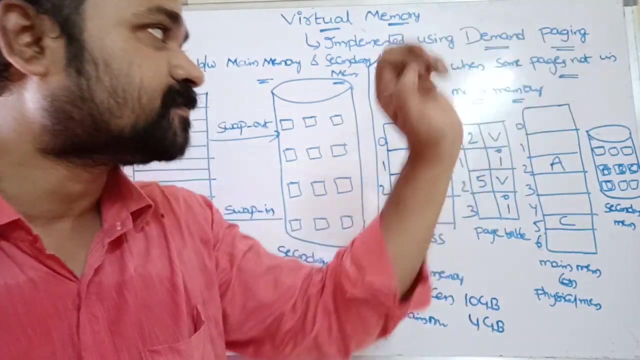 But here demand paging. The name itself specifies the meaning. Whenever there is a demand for the PACE, then only operating system loads that PACE into the main memory. That means CPU will execute a PACE whenever this PACE is resets in the main memory. 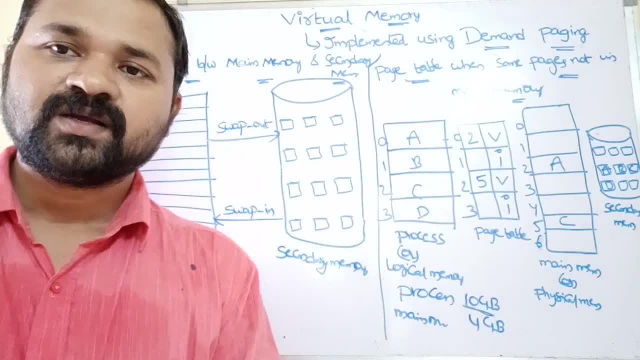 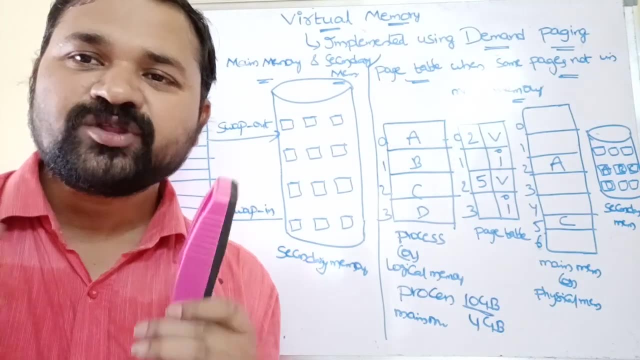 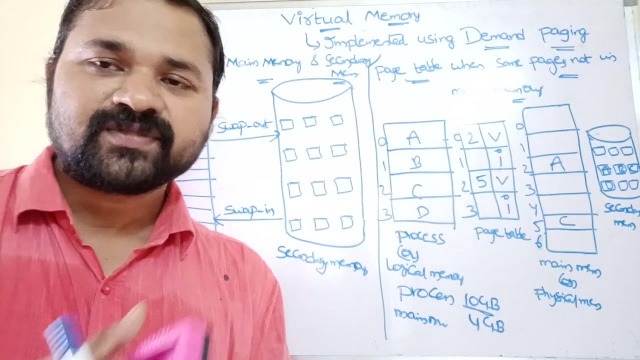 Let. size of the process is 10 GB, But CPU can't execute the entire process at once. We know that at a time CPU executes only one instruction, So depends upon the module. the corresponding PACE that needs to be executed will be loaded into the main memory. 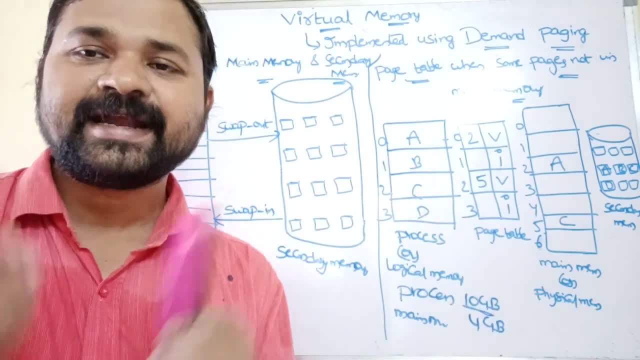 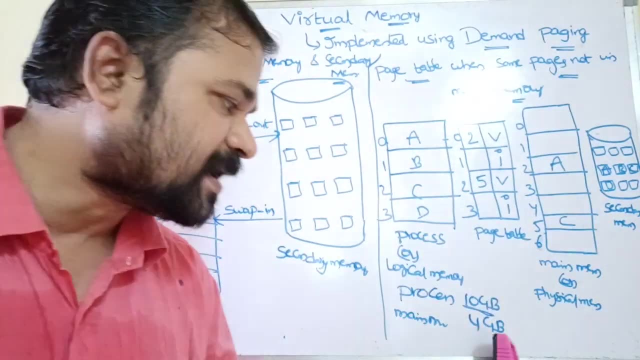 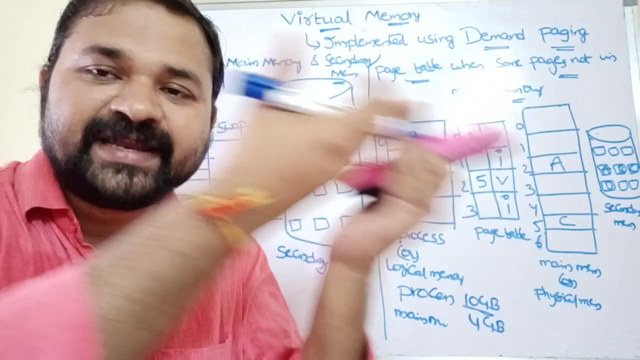 So that CPU executes that instruction. Let us take a movie. Let we are watching a movie whose capacity is 10 GB, Whereas our main memory capacity is 4 GB. Let we are at the first minute of the movie. Then the first minute of that PACE will be loaded from secondary memory to the main memory. 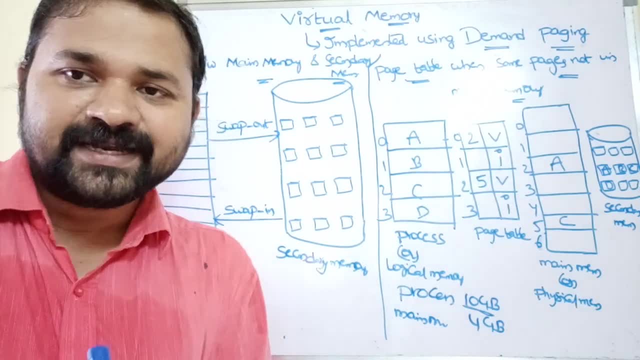 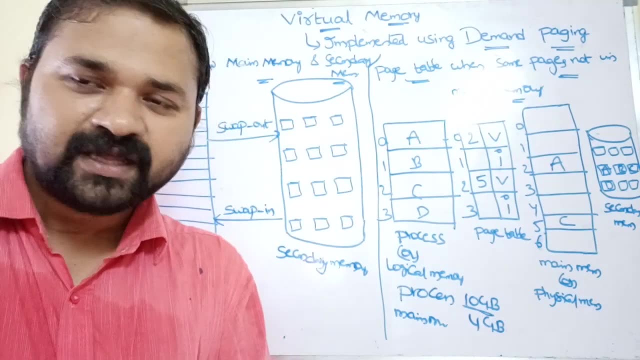 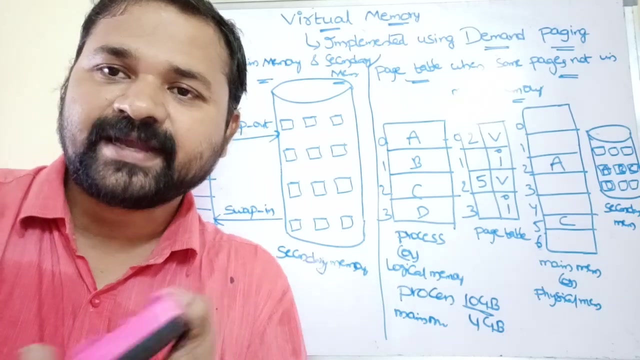 Let we are at 10th minute of the movie. Then the first minute which is available in main memory will be moved to the hard disk And that 10th minute PACE will be loaded from secondary memory to the main memory. Let we are at some interval portion. 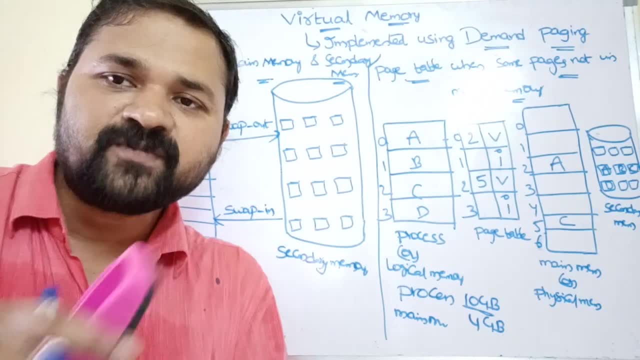 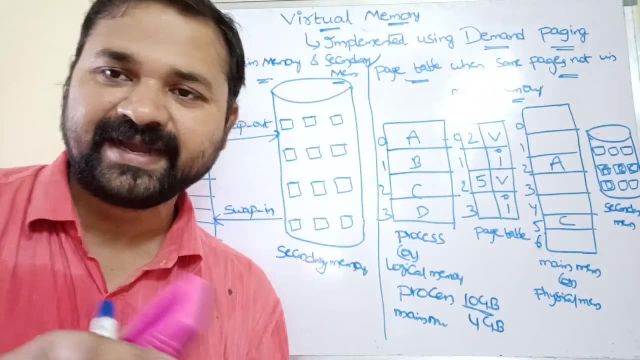 Then that PACE interval, PACE will be loaded from secondary memory So that PACE is loaded to the main memory. So likewise, CPU executes the process depending upon the demand. But here what is the point? at a time, CPU executes only one instruction. 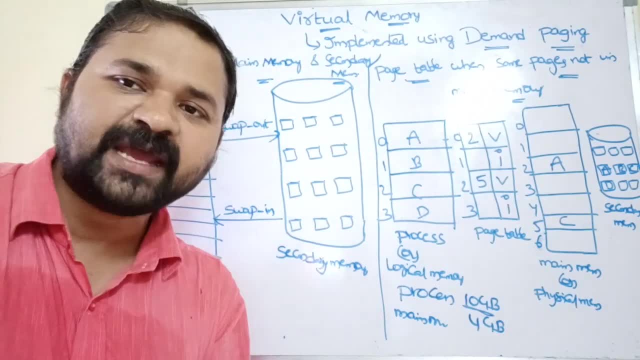 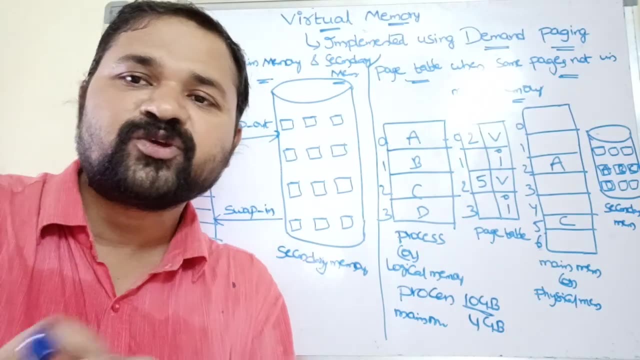 So there is no need to load the entire process into the main memory at once. Depending upon the user request, CPU loads that PACE from secondary memory to the main memory. So that is why this is called as demand pacing. So virtual memory is implemented using demand pacing. 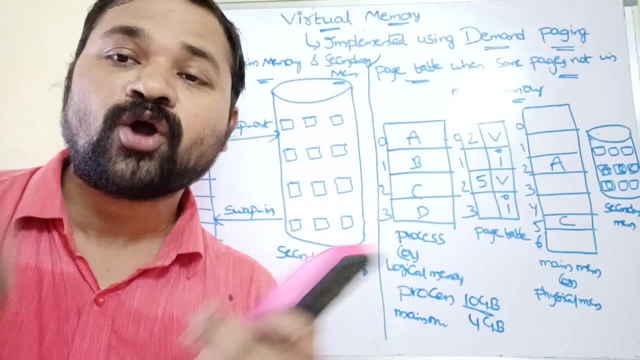 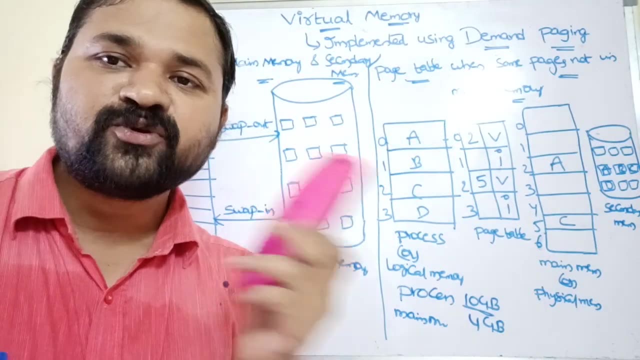 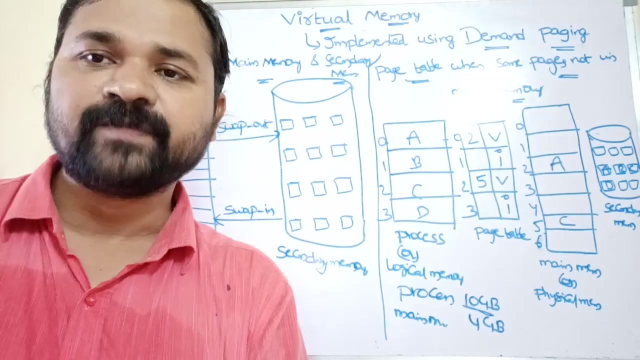 paging here. virtual virtual means not real, it is an illusion. an imaginary virtual memory is an imaginary memory. by using virtual memory we can execute a process even if process size is greater than the main memory. so let's see this now. let's see this diagram swapping between main 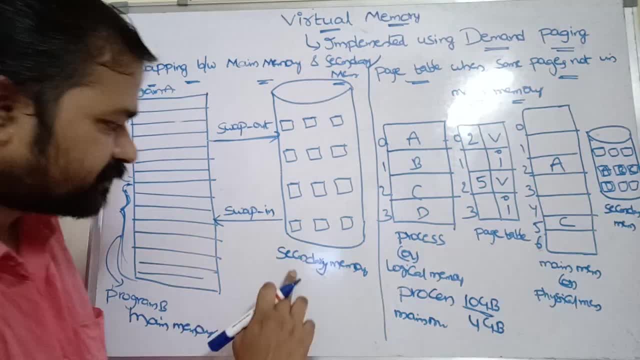 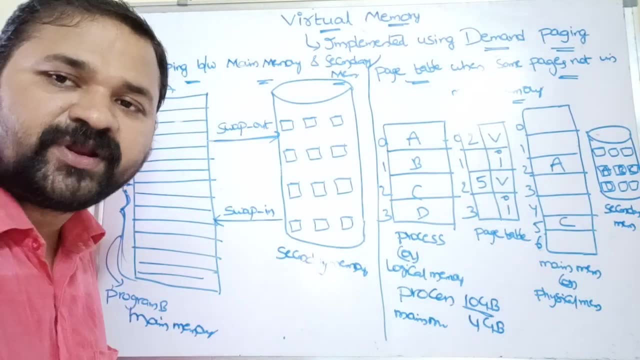 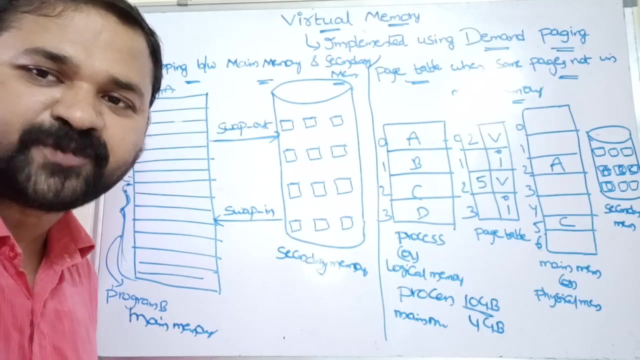 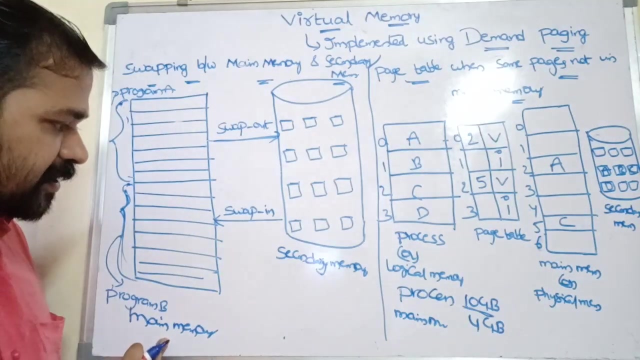 memory and secondary memory. so this is our main memory, this is secondary memory. let us assume that CPU is executing program here. let program here has completed all its operations. so then there is no need of CPU for program here. why? because program here has completed all its operations. then the pages of program here are moved from main memory to the secondary memory. 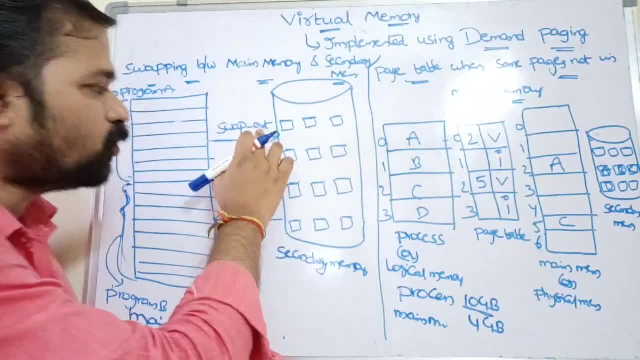 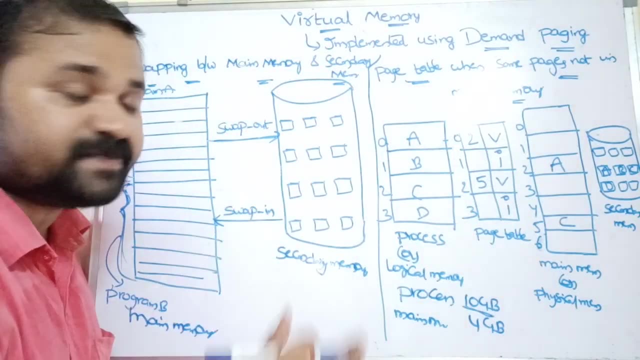 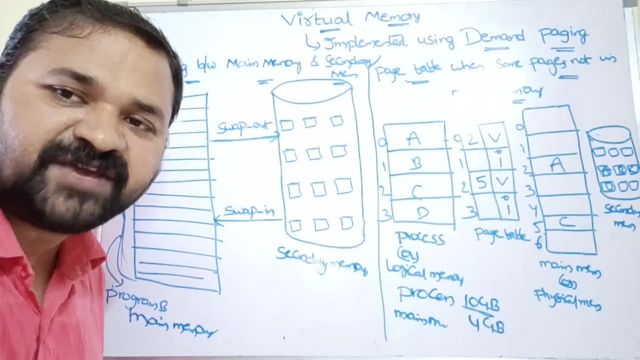 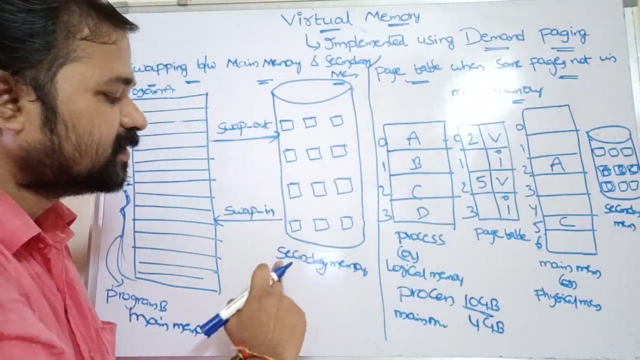 this activity is known as rapport. so swap out means moving the pages of the program from main memory to the secondary memory. and let us assume that CPU is free. that means CPU is ready for executing a program. then operating system loads the pages from are the program from the secondary memory to the main memory. 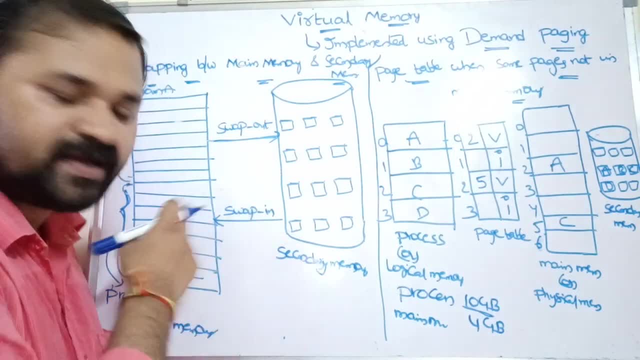 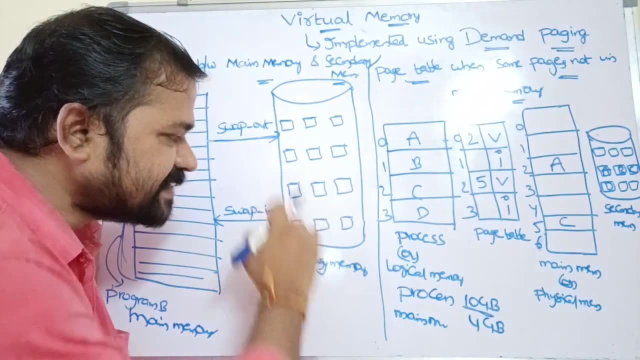 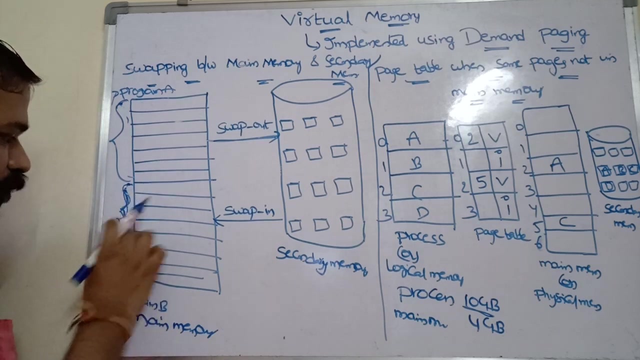 why? because we know that CPU executes a program when it resides in main memory only. so whenever the CPU is free, then the operating system loads the pages of the program from the secondary memory, secondary memory to the main memory. so let it, let. that is nothing but program b. so program b pages. 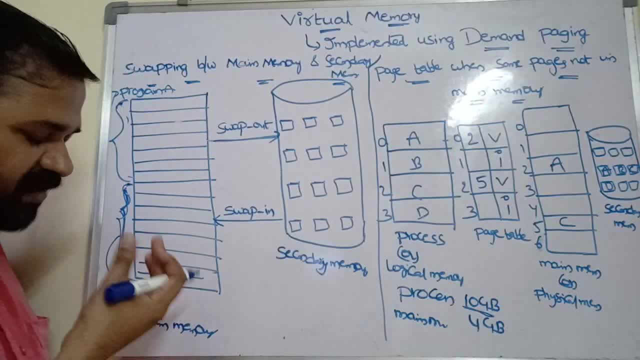 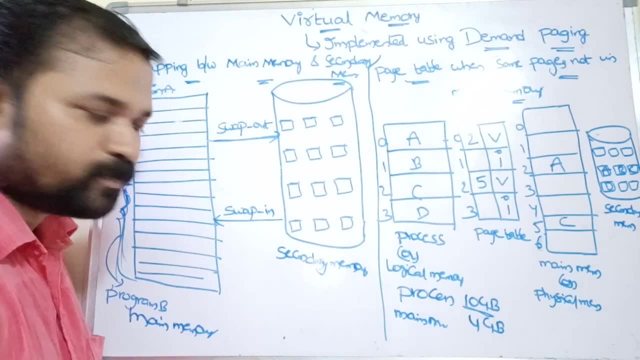 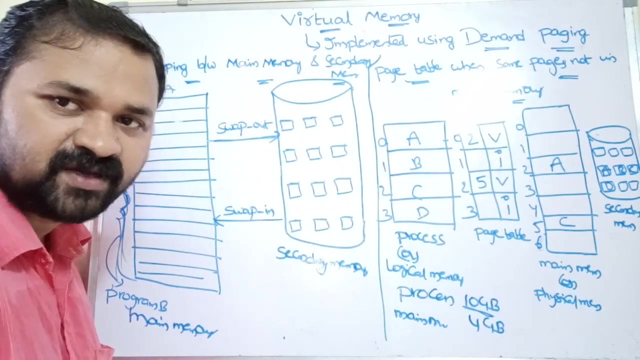 are moved from the secondary memory to the main memory. why? because cpu is ready for execution and this process is known as swapping. so swapping means moving the pages of the program from secondary memory to the main memory. so with this the demand paging will be implemented. so whenever, 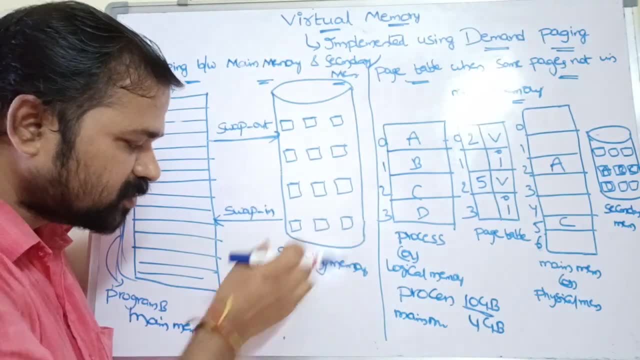 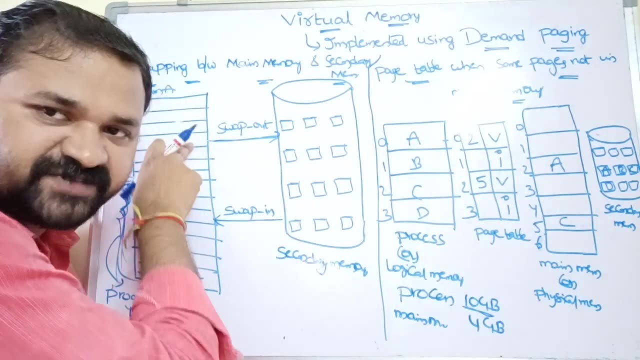 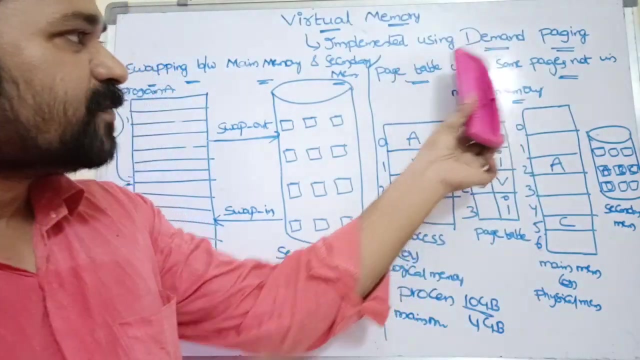 there is a demand for the base, then the operating system moves that base from secondary memory to the main memory. so once that page execution was over, then that pace will be moved from moved from main memory to the secondary memory. now let's see this diagram pasteable when some pages are not in the main memory. so this is nothing but our process, or? 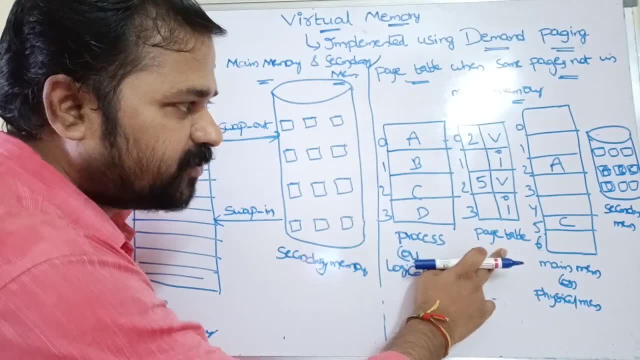 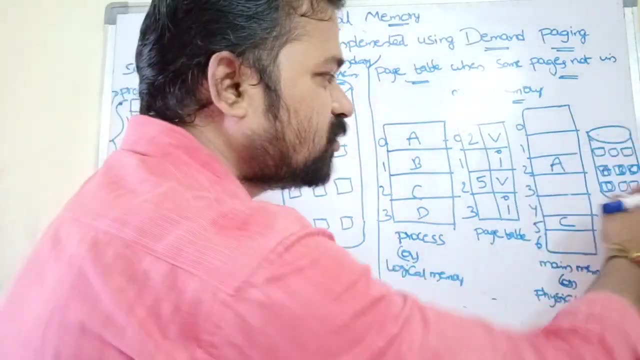 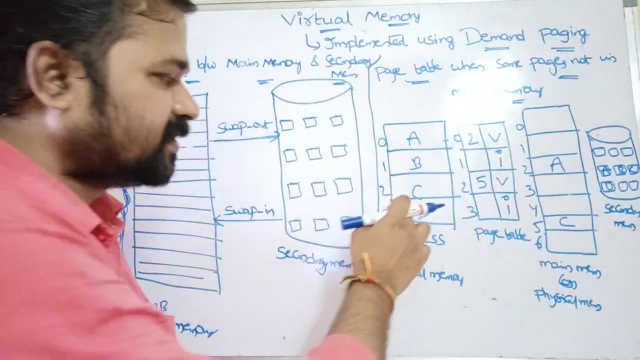 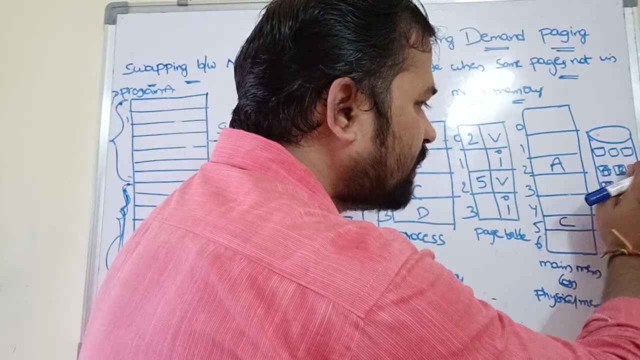 logical memory. this is nothing but pasteable. this one main memory or physical memory, so this one secondary memory. so let initially we know that secondary memory contains a number of processes. let here secondary memory contains process a, pages here. process here totally contains four pages: a, b, c, d. so this a, b, c, d, so a, b, c, d pages are. 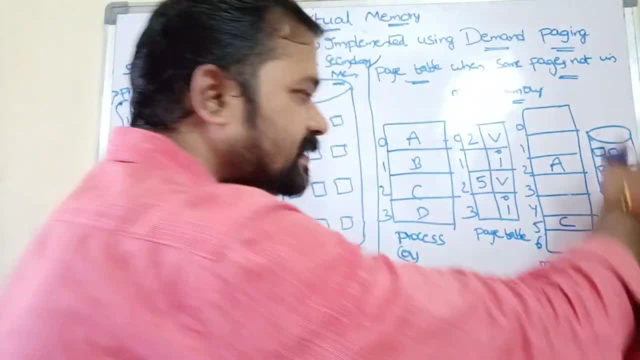 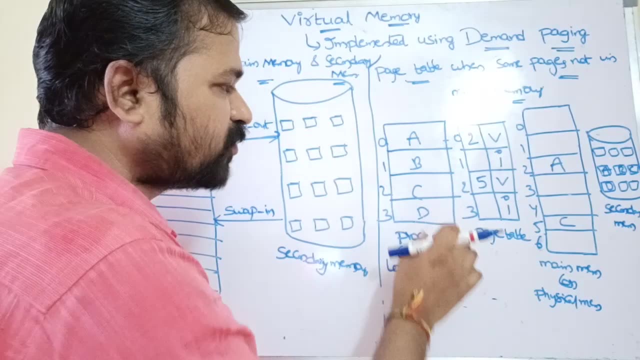 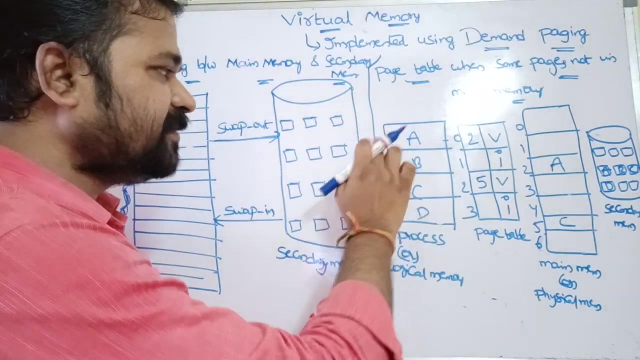 available in secondary memory. in addition to that secondary memory may contains other process pages also. so this is process or logical memory. so totally here, process contains four pages. the first page is a, second page is b, third page c, fourth is d. so a means page number zero, b means page number one, c means page number two, d means page number three. 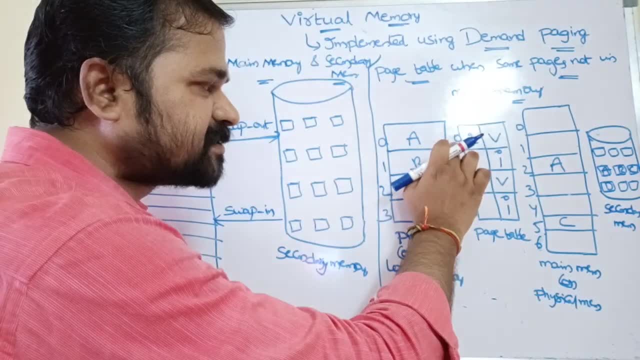 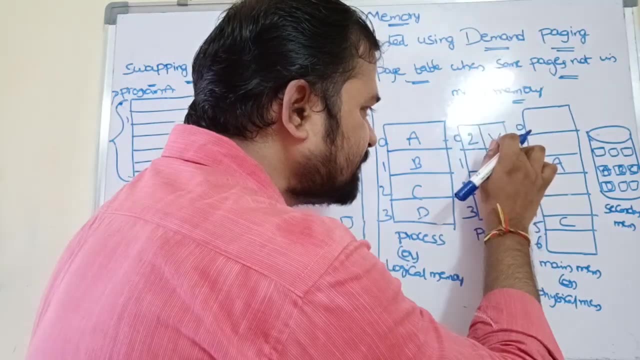 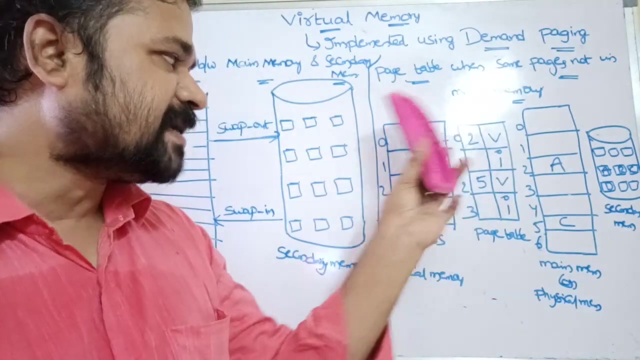 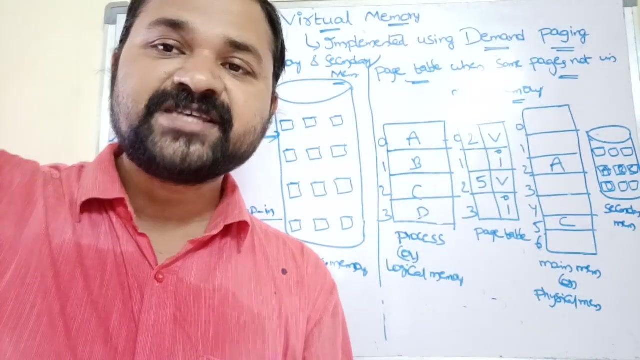 so this is a pasteable. we know that pasteable accepts page number as the input and produces frame number as the output. here for production week we using b and a, v and i in paging concept. v specifies that the corresponding page number belonging to the process. v stands for valid bit, whereas i stands for invalid bit in paging concept. 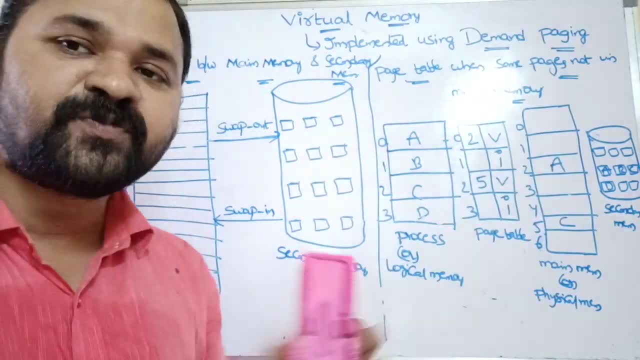 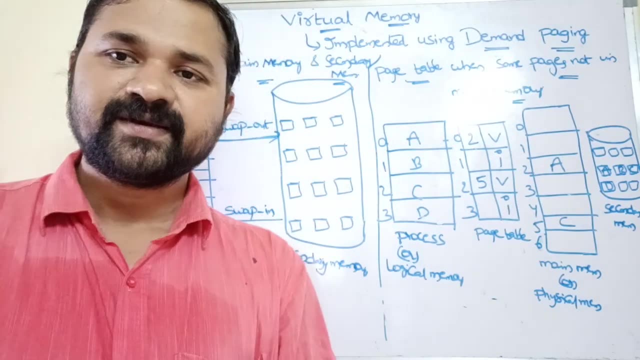 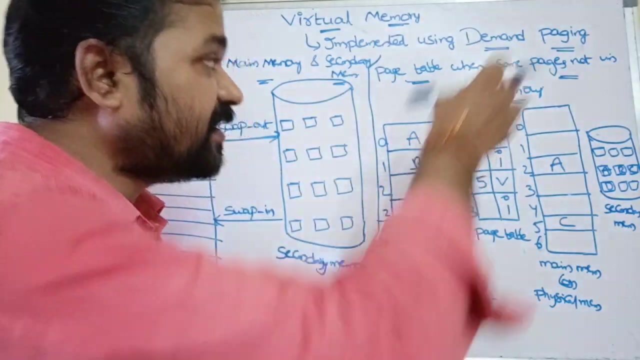 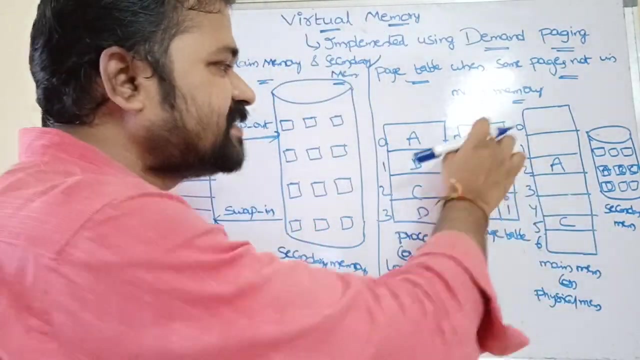 i specifies that this page number doesn't belongs to the process. so in paging v specifies that the corresponding page belongs to the process, whereas i specifies that the corresponding page doesn't belongs to the process. various in paging concept. various in demand paging concept. this v specifies that this page number present in the main memory which stands for valid bit, whereas i stands for. 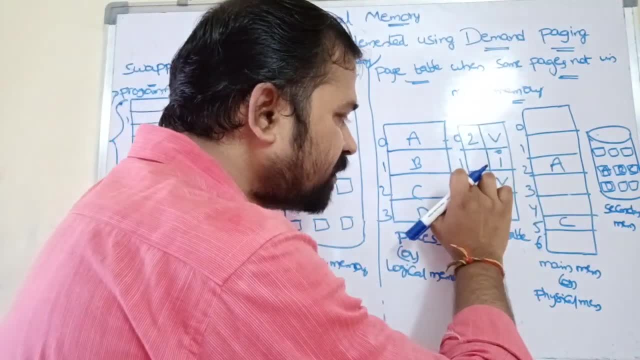 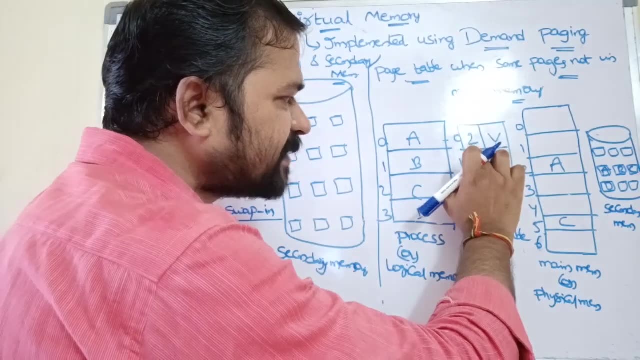 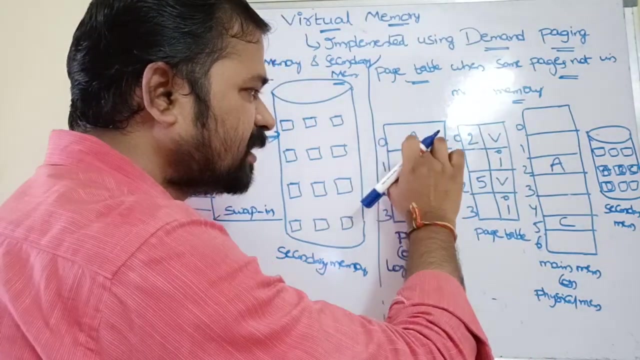 invalid bit. here i specifies that this page number is not present in the main memory. if you observe the first row, it specifies that page number 0 is present in the main, present in the main memory of frame second. so frame number second contains page number 0. page number 0 is nothing but a. 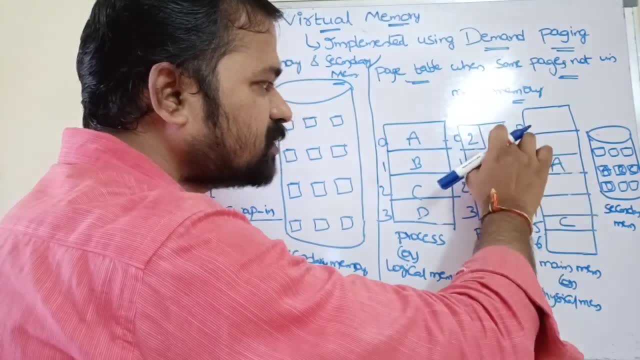 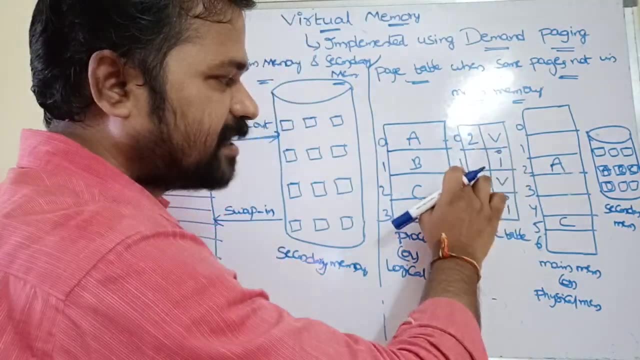 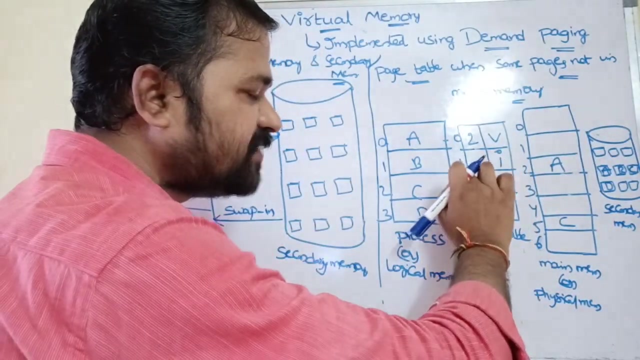 here this page is present in the main memory, so the production bit is valid. v. if you observe the second row 1, here there is no data. that means this page number 1 is not present in the main memory. here the production bit is invalid, so invalid specifies that the page number 1 not present in. 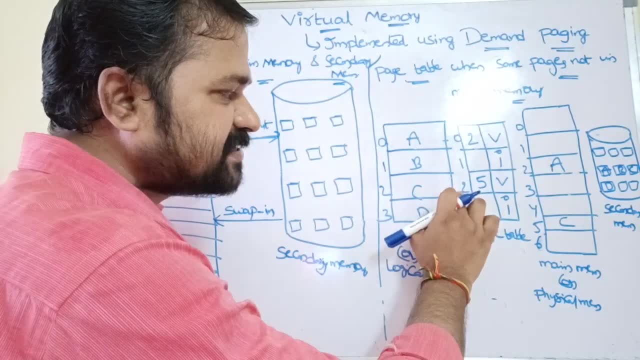 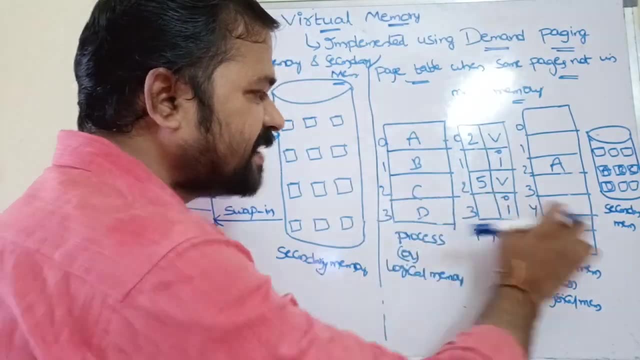 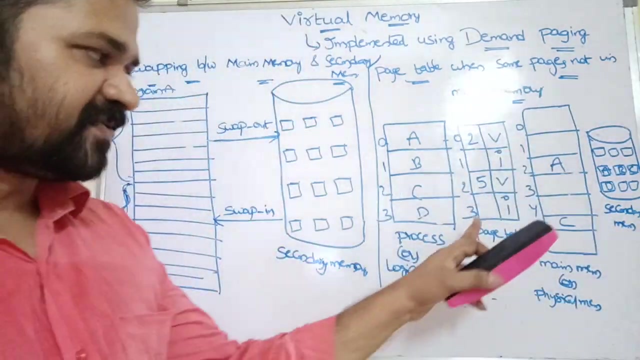 main memory. if you observe this row, it specifies that page number 2, present in the main memory of frame 5, so fifth frame contains page number 2. page number 2 means c, so here the production bit is valid. why? because this page number is present in the main memory, so likewise the last page number doesn't available. 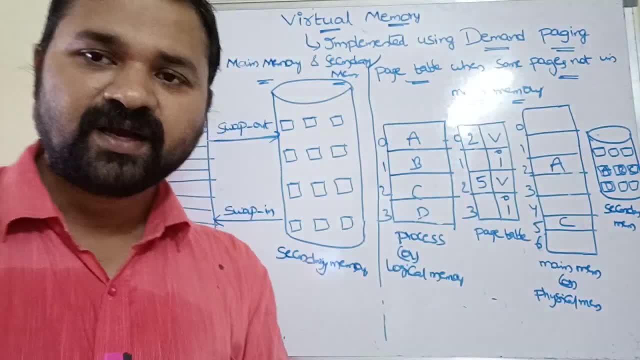 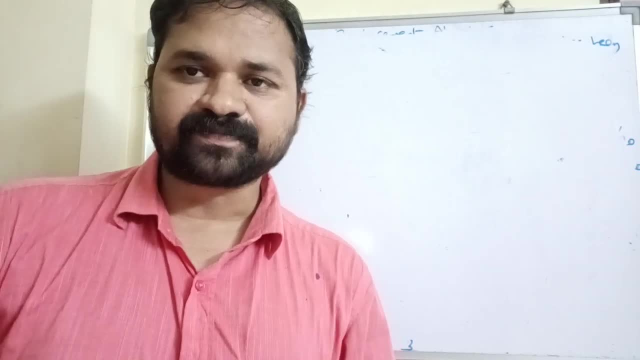 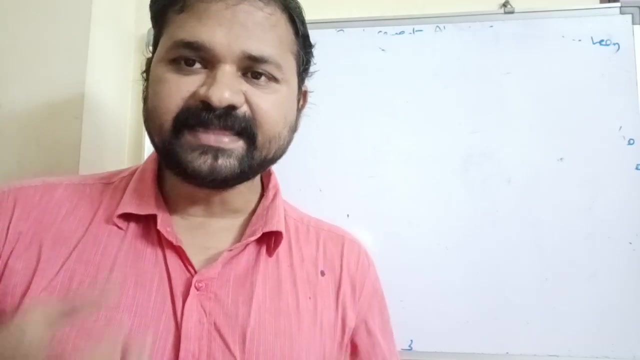 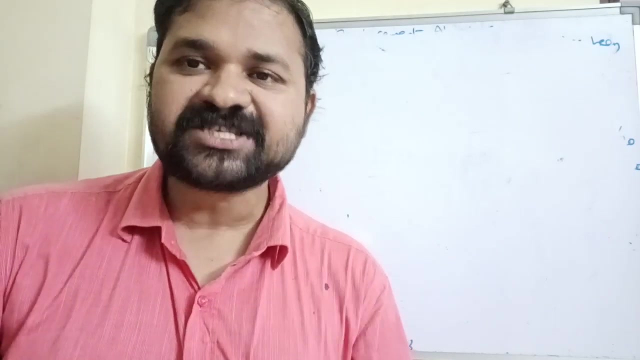 in the main memory. so the production bit is i. now let's see about page fault. when cpu needs to execute a page, then it checks whether that page is available in main memory or not. if the page is available in main memory, then there is no problem. cpu executes that page. if the page is not present in the main memory, then it is called as page fault. 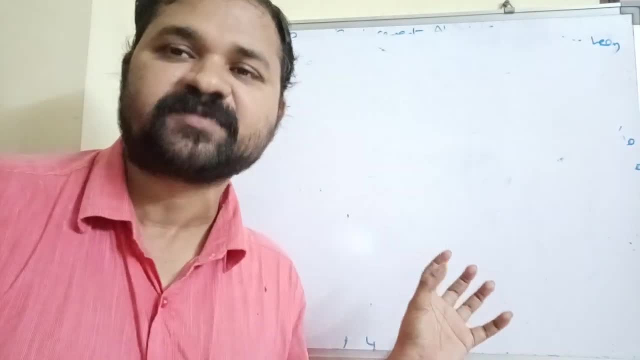 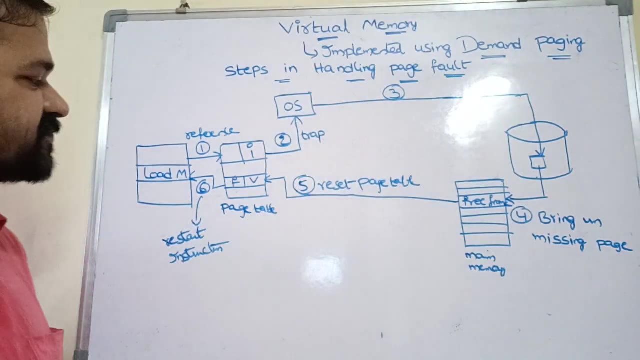 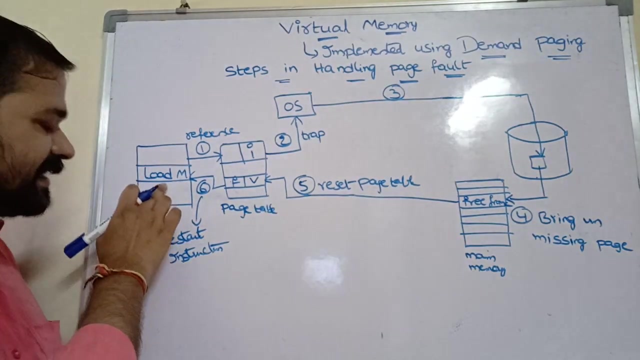 so whenever page fault occur, then we have to perform some steps. let's see those steps now. now let's see this diagram: steps in handling a page fault. let's see the first step here. so whenever cpu needs to execute a base, then it checks whether that page is present in page table or not. 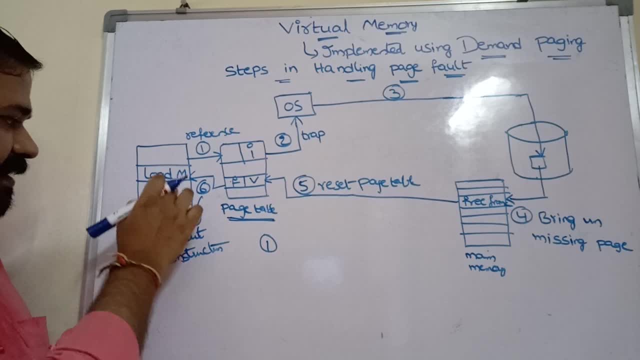 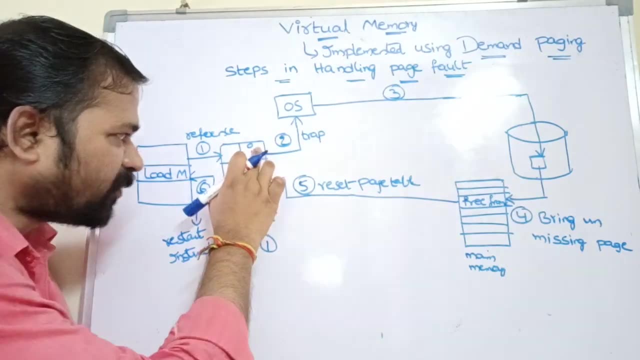 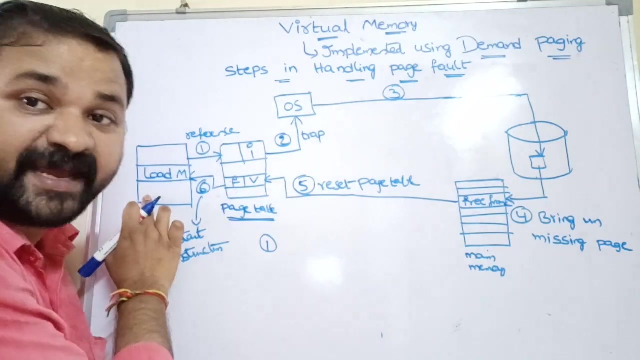 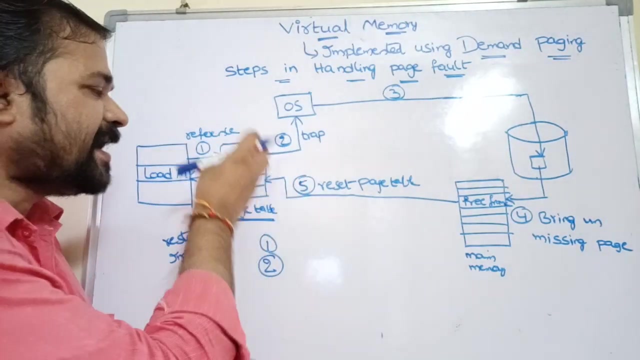 so this is the first step here. here the pare is not present in main memory. so that is the first step. now lets see the second step here. the page is not present in the main memory, so cpu generates an interrupt called speech. 학师的�з小跳 esquer孔. 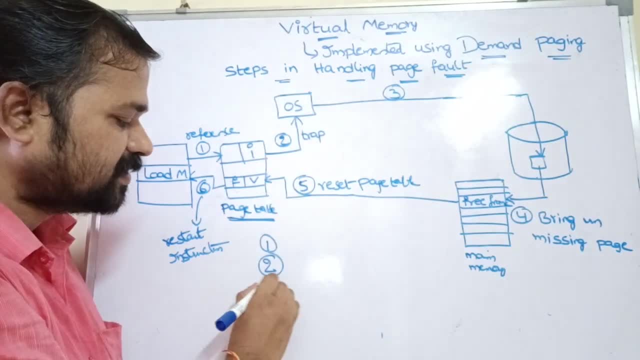 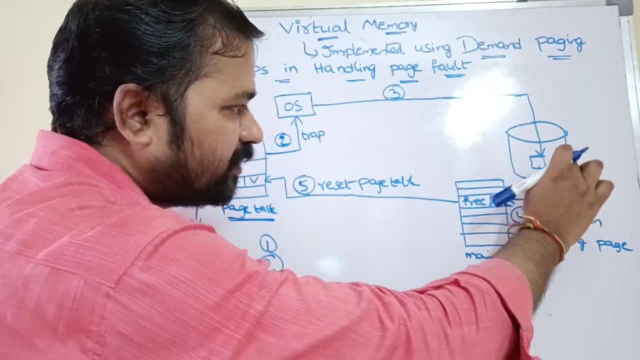 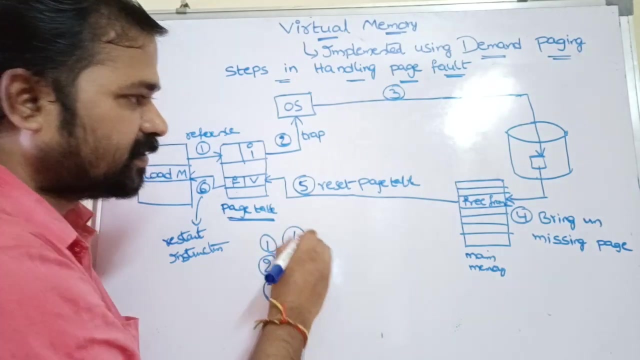 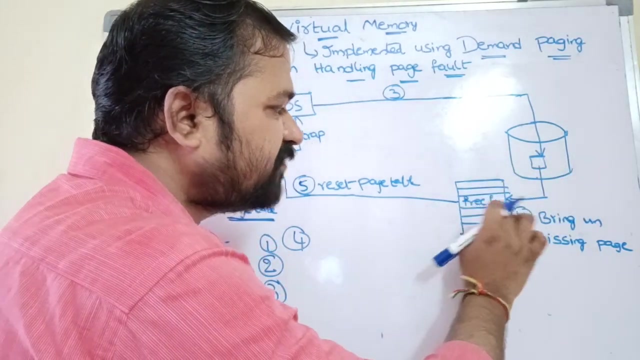 trap to the operating system. this is the second step. next third step: operating system checks where that page is present in the secondary memory. so this is our secondary memory. so it checks where that page is present in the secondary memory. next fourth step: operating system loads that page from secondary memory to a free frame of the main memory. so this is the fourth step. 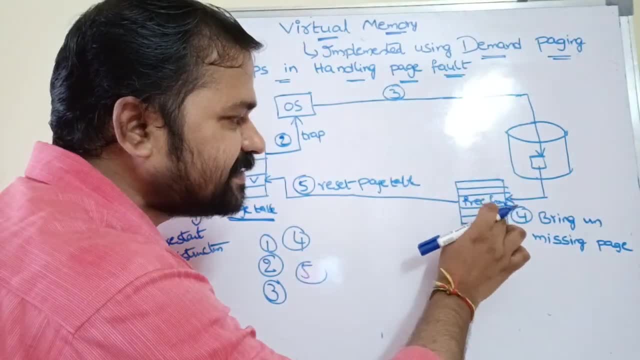 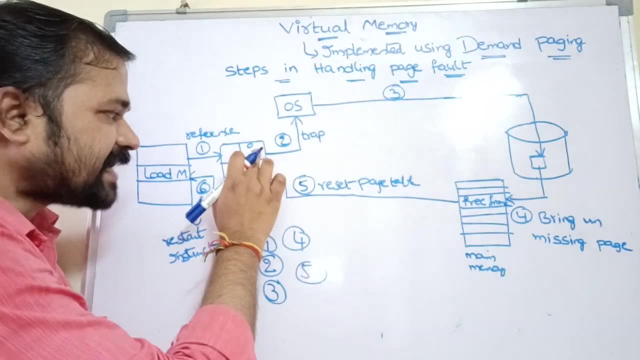 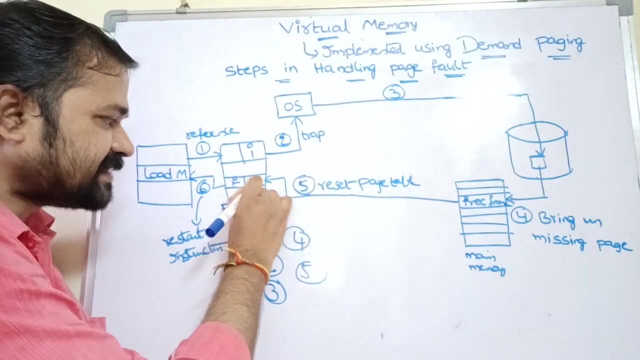 now our main memory contains the corresponding frame, so we have to change the production bit here so we can change as this: i should be changed to v. why? because now the page number is present in the main memory. next, as well as this frame number, information will also be specified here.